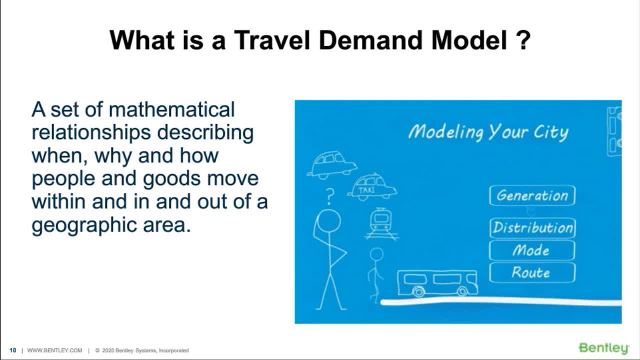 we call a four-step model approach. The first step is trip generation, second is trip distribution, then mode choice and finally route choice. The geographic area may be a small area of the CBD, Or an entire city or a metropolitan region, a state, a country or even a multinational region. 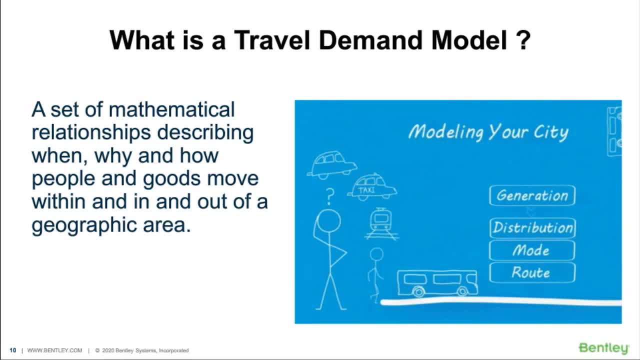 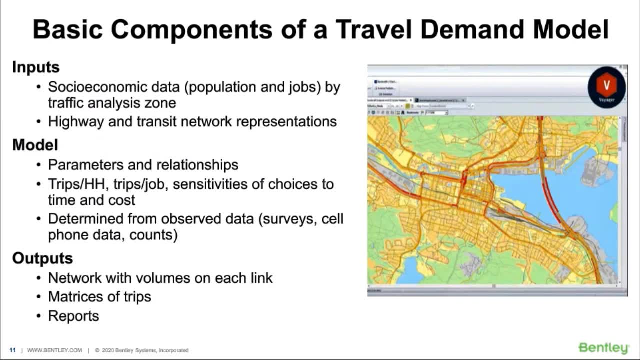 such as region along the Mekong River Delta and so on. There are three basic components of a travel demand model. Number one is the input, and the basic input into a travel demand model is social economic data, mainly population and employment. population and jobs by traffic analysis. 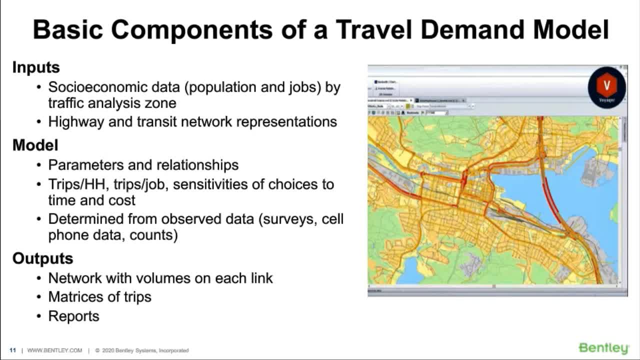 zone. Typically we'll divide up the study area, either the city or a state, into what we call traffic analysis zone And we need population and jobs data from for each of these zone, And typically these are coming from the planning department. The second major input that is required for a travel demand model is highway and transit network. 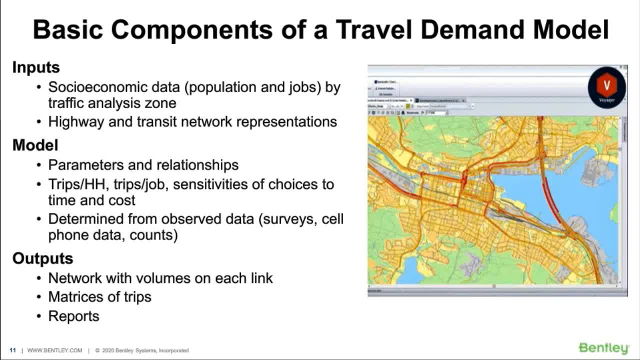 representations. We devise a way of representing highway network and bus network, metro network in the computer. The model itself is a set of parameters and relationships describing how people make trips, And, for example, some of these parameters are number of trips produced per household or number of trips produced per job. 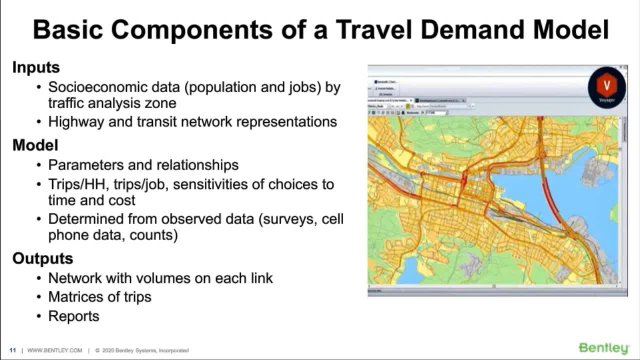 And the model. the relationship also includes sensitivities of choices to time and cost, how people choose between different mode, including walking, biking, driving along, carpooling or taking the bus, taking the metro, things like that. And if they all, if they decided. 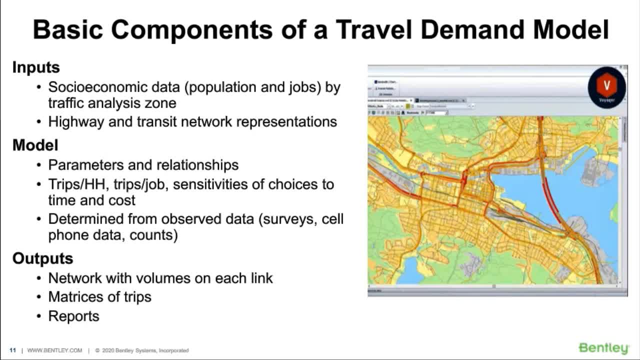 to drive? which route would they take? These are a set of relationship describing the sensitivity of choices over time and cost. And how do we know? we're doing a good job in kind of modeling or simulating the reality. So typically, a lot of data will be required from the observed data We'll have. 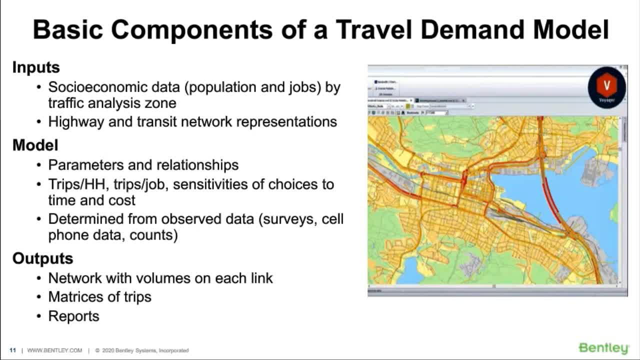 household survey, cell phone And nowadays we actually got a lot of data from the cell phone data to use those as observed data to calibrate. to see how good we are, Excuse me, To see how good we are doing with all the modeling that we're doing. The outputs from the travel demand model that we're looking for is network with. 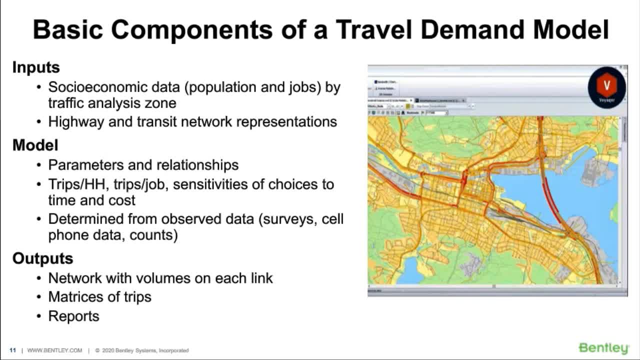 volumes on each link. this is a measurement for us to see how our infrastructure are doing in terms of meeting the travel demand. where the congestions are, do we need to widen certain roadway and bridges? do we need to construct an entire new freeway or do do we need to have more buses or 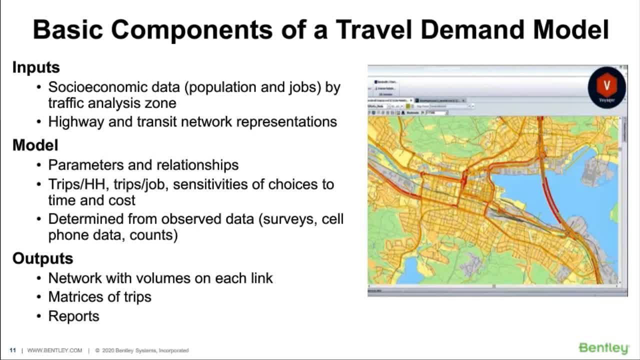 metro lines. so these are the, the output that we mainly are interested in doing travel demand modeling. a byproduct, very important byproduct, of the model is what we call matrices of trips, commonly referred to as od tables, because, remember, we, if we divided up the entire city. 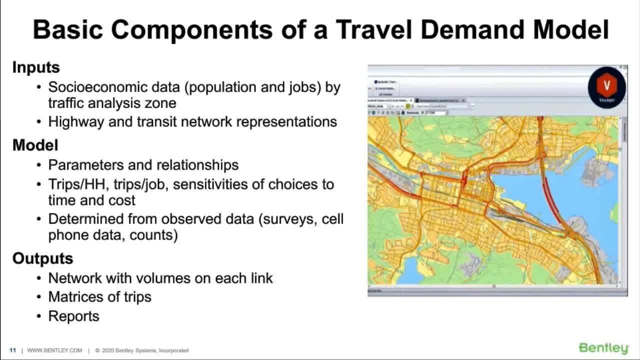 in 1 000 zones, then we'll be able to see 1 000 by 1 000 metrics of how many people going from zone 100 to zone 201 and so on and so forth, and that is a very good information in terms of giving us an idea of the travel patterns of your region. 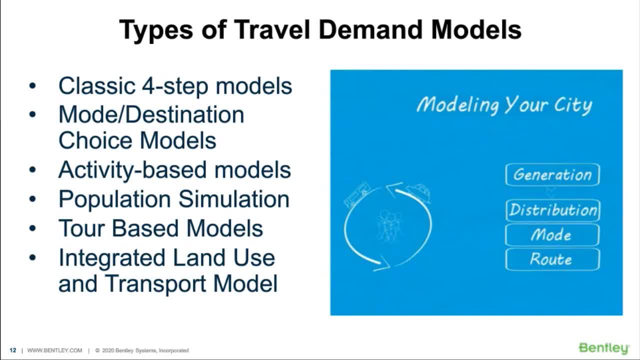 besides the four-step models that i mentioned earlier- trip generation, distribution, mode choice and route choice- there are several other more advanced models that we can use to understand the travel patterns of your region. so, in order to step into the model, in terms of those four-step models, our benchmark is: 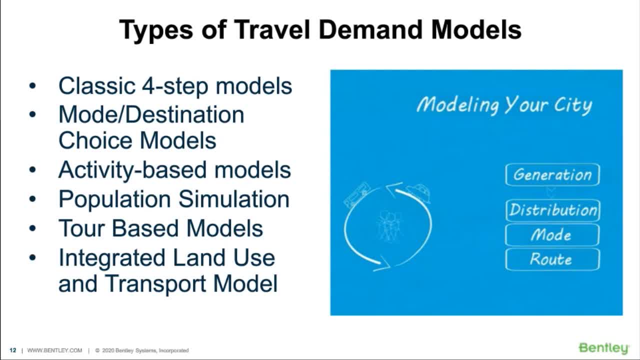 incredibly router advanced, so we also modify the last three semaines or so we start at each league transitioning, and that includes other different models on top of our friedgeb and abstracting their active design and combat performance. now, right now, we are in the sense of the travel petroleum. date is 11 March and it's all about november 15, and it's still. 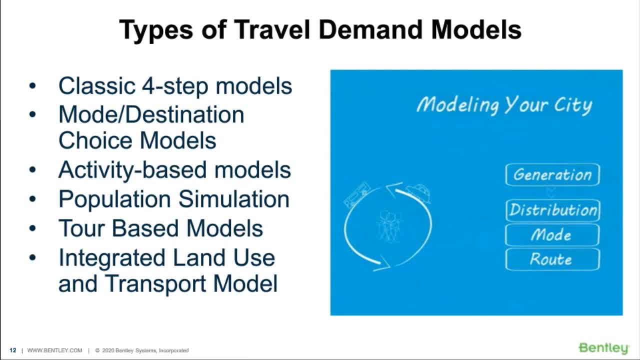 12 May and it's coming down to the laptop year and Dan is correct and they must turn off the acquit date, so maybe we have a face time studies by the end of 2017 computer. so we now need myths are listed seats 6 months so and that takes kind of the. 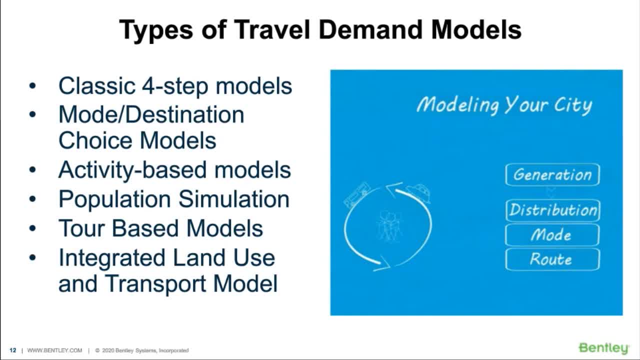 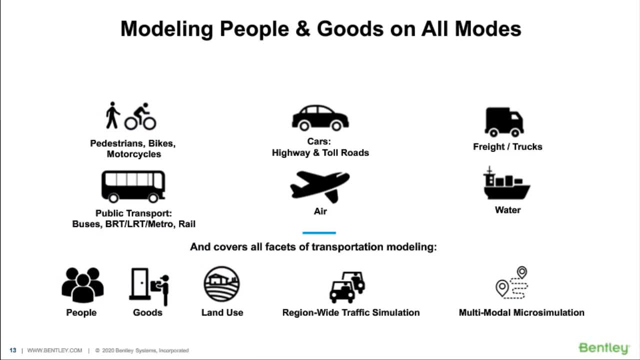 question why we should let you know what that means. what model we create now ones is it's a perceptual model. this is yuan growing industry and they spending 100 dollars 205. so a dassel travel demand models may be built to model all or some of the most shown on this slide. 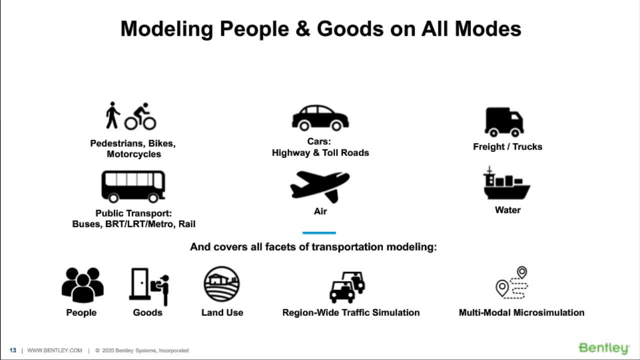 depending on the purpose of the project. so if it's a bicycle model, so now you will have a bicycle mode in there, not most. most of the regional model or models for travel for metropolitan area they probably only include cars and public transport may not necessarily have the 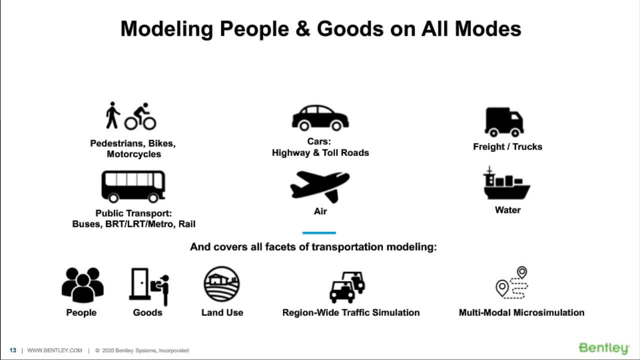 pedestrian and bicycle or motorcycle in there. national model, that that need to look at the movement of people and goods in the country or in and out of the country. then air mode sometime will be included too. there are three levels of modeling. on the top is what we. 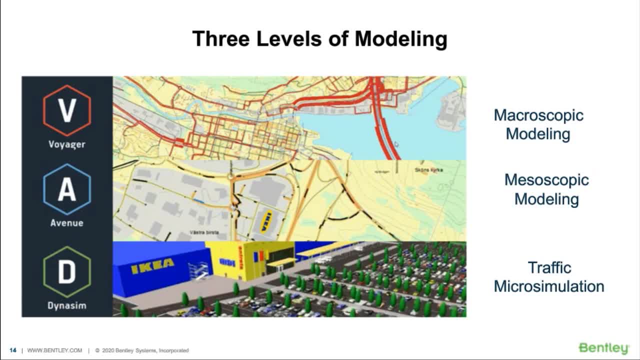 refer to as a macroscopic model, which is mainly for understanding travel pattern and assessing the need for transportation infrastructure, such as highways and public transport. the next level is mesoscopic level modeling. this level of modeling allows transportation planners to analyze traffic congestions and queues over time, especially during peak periods. and finally, there is a traffic simulation. 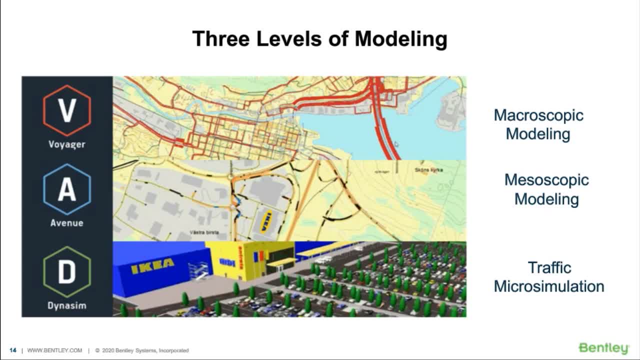 the microscopic level of modeling. at this level, traffic engineers can lay out every details of the road and junctions of a study area and simulate the movement of individual vehicles and pedestrians. the cube module for macroscopic modeling is called voyager and the module for a macroscopic modeling is called cube avenue, and our traffic microsimulation module is called cube. 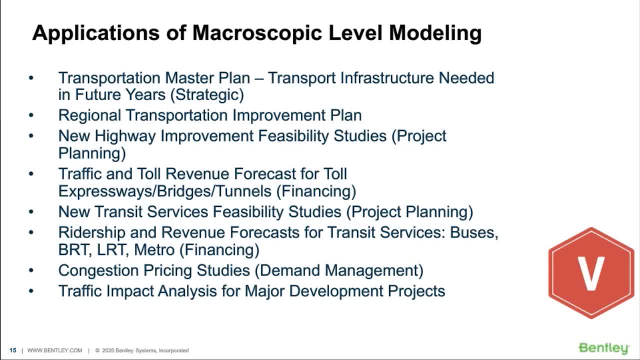 dynasim. now let's talk about why people do travel demand modeling. major application of macroscopic level modeling are the following: number one: transportation master plan. this is to look into the transportation infrastructure network. summary of transportation infrastructure needed in future years. at the more strategic level, 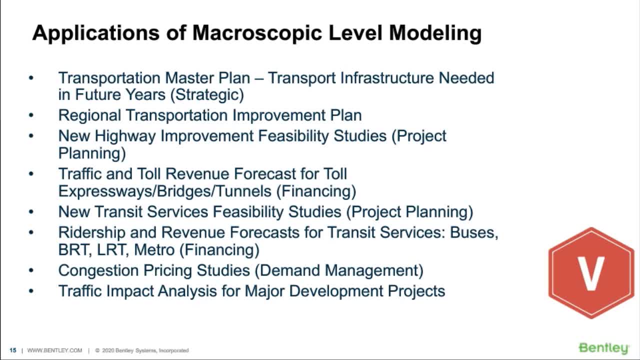 Many states, DOTs, many nations will have a national transportation master plan or state transportation master plan, and that is for this level of modeling. And secondly, regional transportation improvement plan. Well, the first one, the master plan, may be looking to at least 20, 30 years down the road. 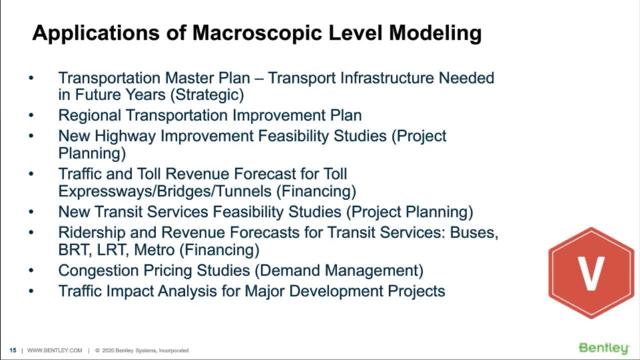 And the regional transportation improvement may be for 5 to 10 years. actually looking at the region, looking at the metropolitan area, what kind of project, to what level of implementation for infrastructure that we need to start implementing? And the next type of study will be new highway improvement. 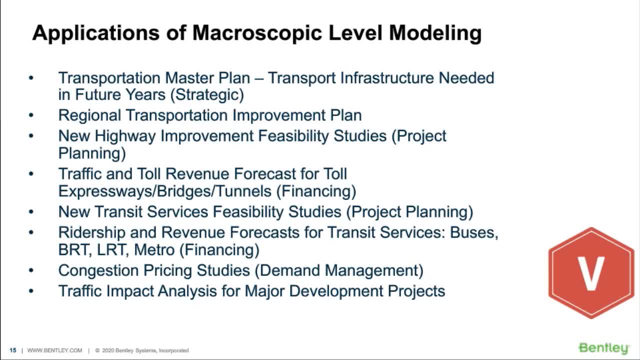 feasibility studies. Now we are talking about. We're talking about individual project level. now, When we design, or before we construct, before we designed a new expressway, for example, we would typically do this type of feasibility study to see what the alignment should look like. 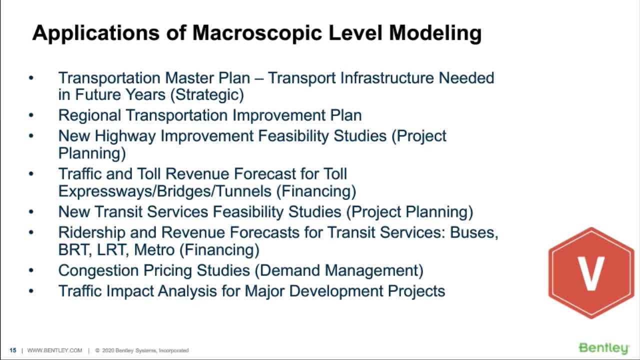 where do we need to have interchanges and the traffic volume requirement that would decide how many lanes, that would describe the interchanges, Interchange layout, that sort of things. And next type of application is for traffic and toll revenue forecast for toll expressway bridges and tunnels. 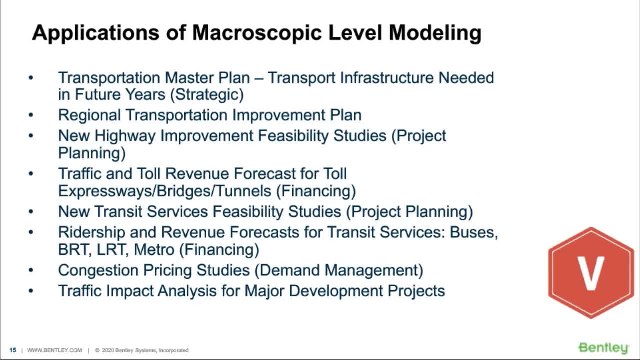 These went beyond the feasibility study. These types of studies typically are done for financing purposes, to looking at how much revenue can we, can an investor, for example- expect from investing on these toll roads? Personally I have done in my career at least 25,. 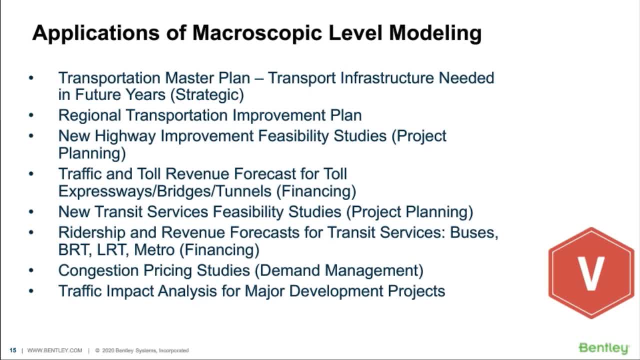 close to 30 toll road projects in the US, as well as in China and Asia, for investors looking at whether this toll road is worth investing or not. So that kind of study is more rigorous in terms of the number and the revenue that is generated. 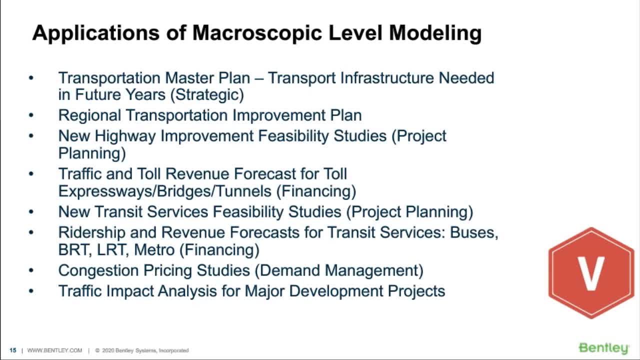 because it's mainly for the financing purposes. Now the application also similar application are also for the transit projects, For example, new transit services, feasibility study, again at the project planning level, And these could be for BRT, LRT, Metro. 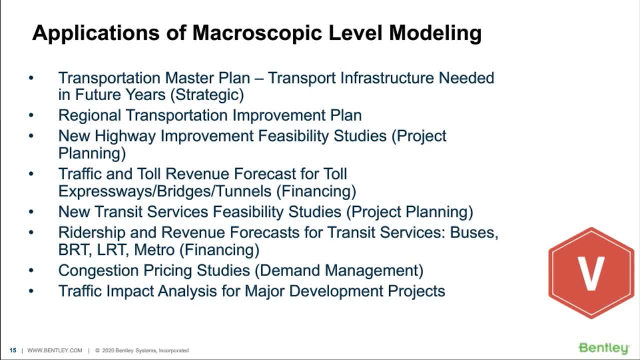 And then likewise, just like toll road ridership and revenue forecast for transit services for financing purposes- Buses, BRT, LRT, Metro- for the financing purposes, And next type of application is more on a demand management side, rather than providing additional infrastructure. 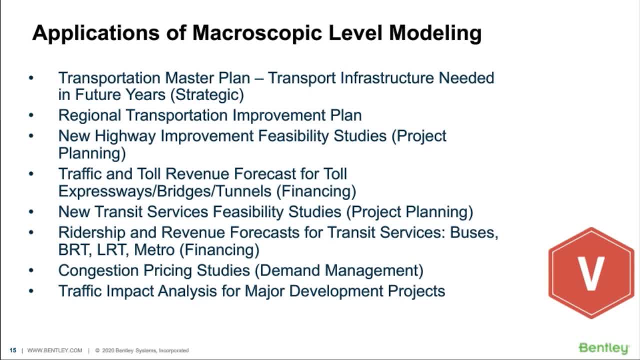 Congestion pricing studies are looking into how to price the existing road Roadway capacity in a congested area, normally CBD, in order to control, to manage the traffic flow inside the congestion pricing area And most of you probably familiar with Singapore. That is the first city in the world to implement congestion pricing And a few years ago London has also done the same And Hong Kong has also studied, done a couple of, for a couple of times they have looking into congestion pricing for Hong Kong. 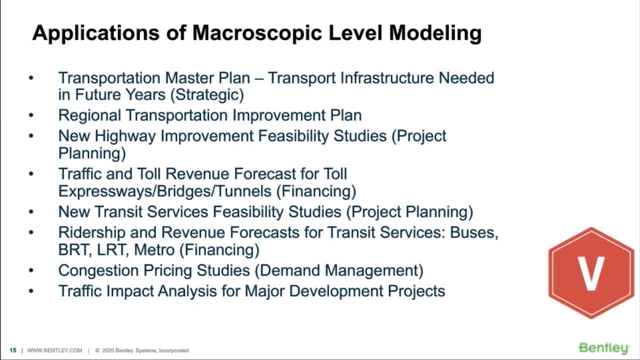 And I have personally participated in one of those study in the late 90s. And the last application on the macroscopic level is traffic impact analysis for major development projects. This could be a development of a new town or redevelopment of an old part of the city or bringing 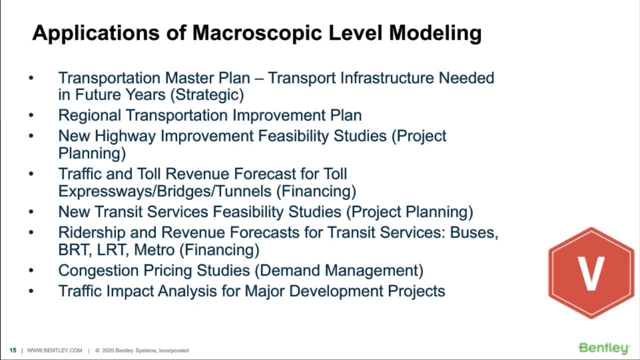 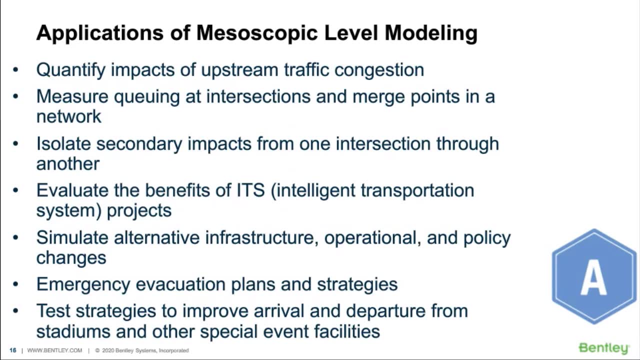 into a major development project for commercial residential. So typically we'll use travel demand modeling for that development area to looking into the traffic impact Application of macroscopic level model. I probably need to speed up a little bit Again. these are the at the macroscopic level we 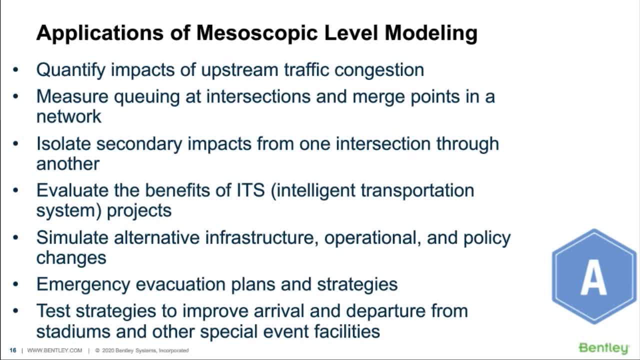 typically people would use the macroscopic level travel demand model and give it more detail and especially introducing time component. One distinction between the macro and the meso is macroscopic modeling is static. We're looking at the average condition of a day or a peak period of a day. 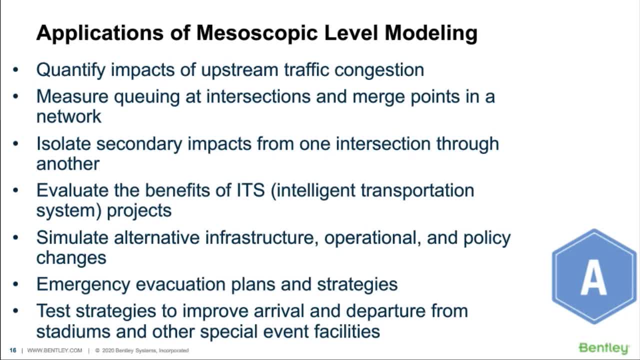 But at the mesoscopic level we will introduce time component. So we're looking at the average condition of a day or a peak period of a day, But at the mesoscopic level we will introduce time component. So we're looking at the average condition of a day or a peak period of a day, But at the mesoscopic level we will introduce time component. 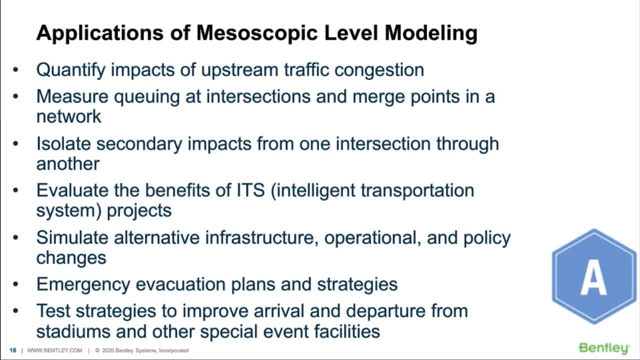 And to do dynamic traffic assignment. So in this case it would allow us to look into the impact of upstream traffic congestion. We can measure queuing a intersection and merge points in a network. We can isolate secondary impacts from one intersection through another. 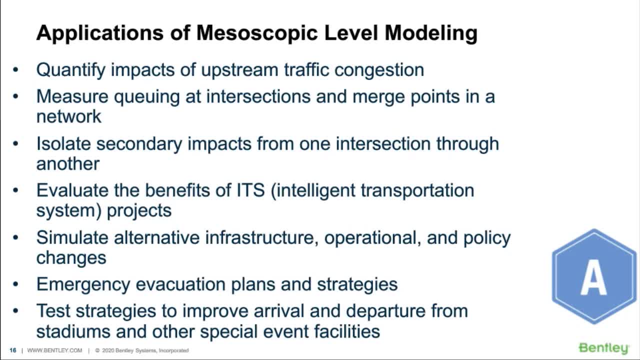 And in order to analyze ITS intelligent transportation system projects, you will require a mesoscopic model. And in order to analyze ITS intelligent transportation system projects, you will require a mesoscopic time-sensitive dynamic modeling. We can also simulate alternative infrastructure, operational and policy changes and emergency evacuation plans. 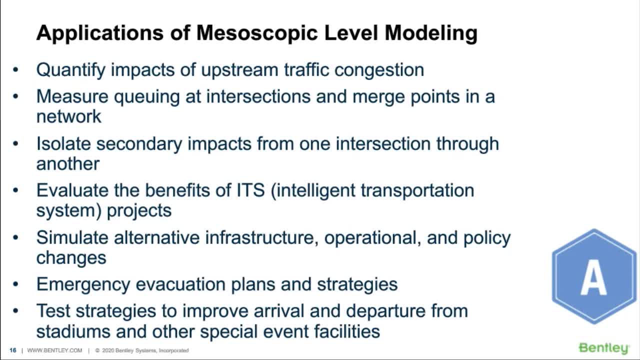 and strategies: Test strategies to improve arrival and departure from stadium and other special events facilities. The last two bullets essentially is describing whenever there's a lot of people want to go to the same place at the same time or a lot of people leaving the same place at the same time.